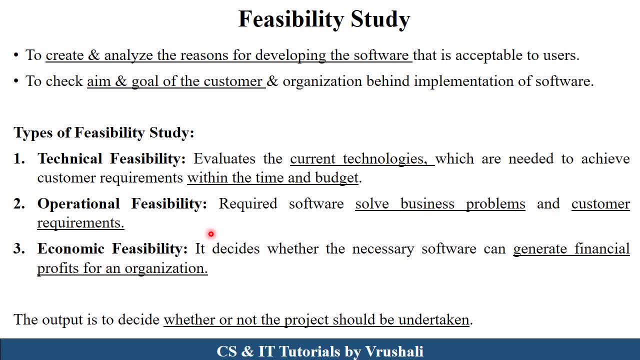 problem. or they complete a customer requirement or not. and in economic feasibility, here the company would develop a product, or company would develop a project. who has a financial profit for an organization or not. so this all three types of feasibility study done here. after that they decide whether a particular project should be developed or not, a particular. 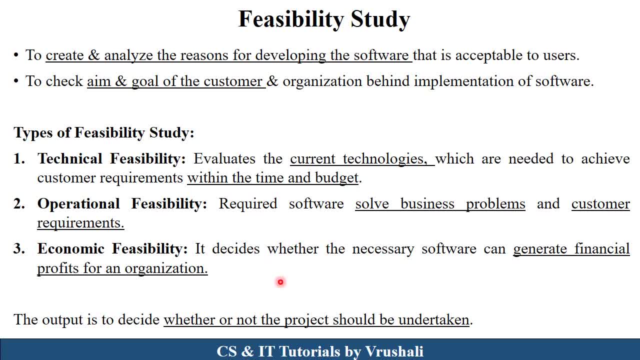 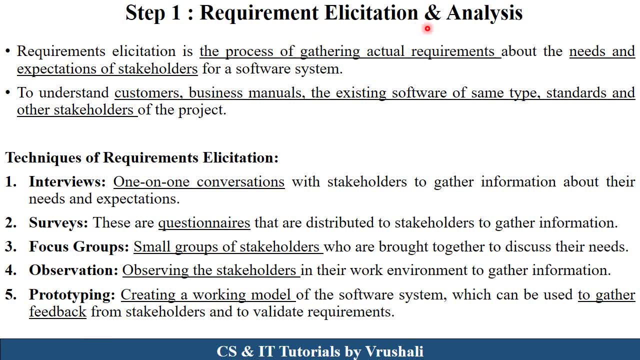 project should be taken first from the customer or not. so this is called as feasibility study. now the next first step in requirement engineering process is requirement elicitation and analysis. basically, requirement elicitation means to gathering all the actual requirements from the customer to analyze need of the customer and what exactly customer want here. in this process they also understand 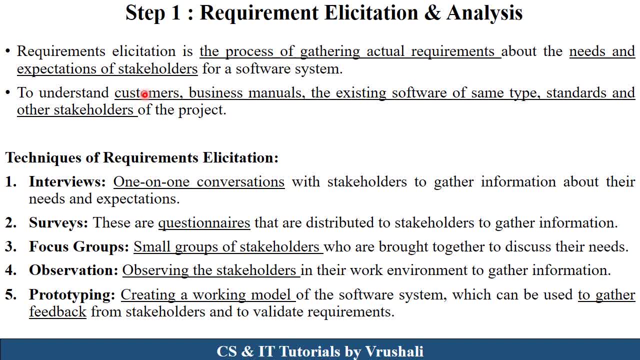 which type of customer, which type of organization use this particular product. business manuals then, suppose customer one college management system application, so this kind of existing software is available or not. the standard of the product and other stakeholder details. so this, all things are analyzed in this particular process. now, this requirement, elicitation having different 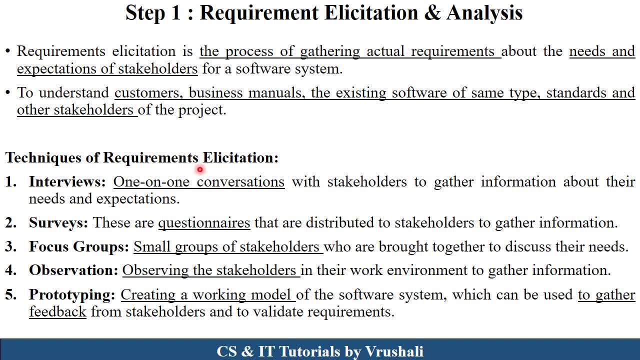 methods here project head conduct different requirement elicitation method to gather requirement from the customer. let's take an example: suppose a particular organization want college management system application. now here project head conduct interviews means one to one conversion with the stakeholder. for example, they conduct one to one interview with principal, different. 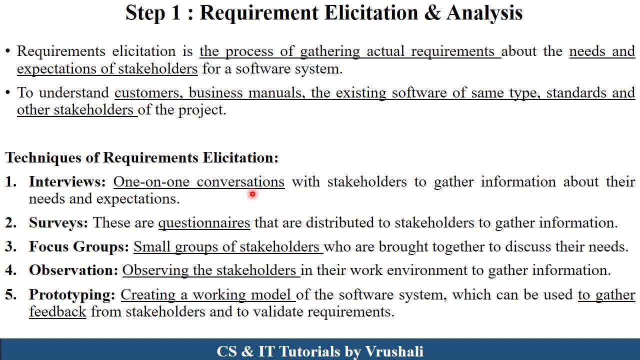 HODs, different teacher staff as well as student. they conduct what exactly customer want, which type of features they want, and they collect the requirement. the second method is survey. they collect questionaries and distribute those questionaries to each and every stakeholder, each and every person, and gather the information. 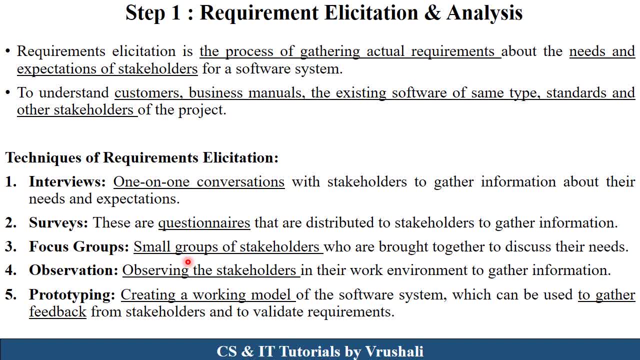 after that: focus on group. here small group of stakeholders means small group of principal, teacher, student and all the other people. they discuss with them which type of functionality they want in particular. project means: teacher want which type of feature, student want which type of feature. this detail. after that observation: here project head observe complete work environment. 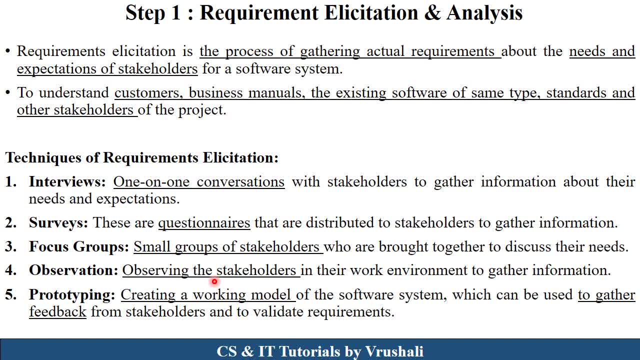 of particular college, particular organization, like which type of colleges are there, which type of particular events are there. so they observe all those thing and at the end they create a prototype. they create a some rough model and as per the customer requirement, and they give this. 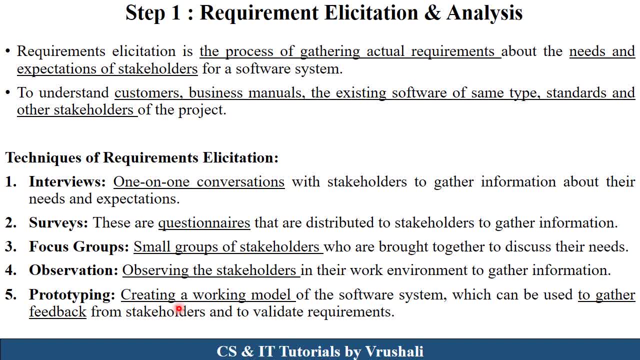 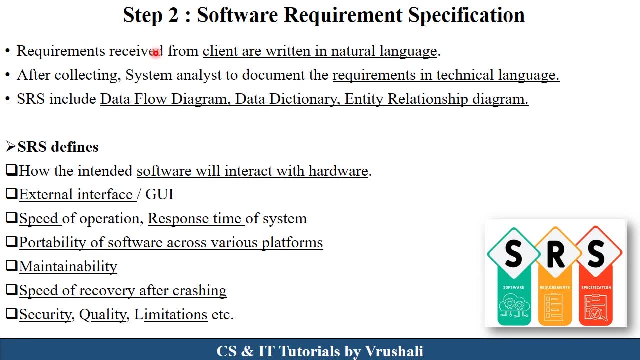 model to the customer. if customer want any changes, they do this changes and after customer satisfaction they develop a actual product. so these are the different methods to collect requirement from the customer. now the next one is a software requirement specification after collecting requirement from the customer. here, system analyst, system analyst- maintain all this requirement in one document. this 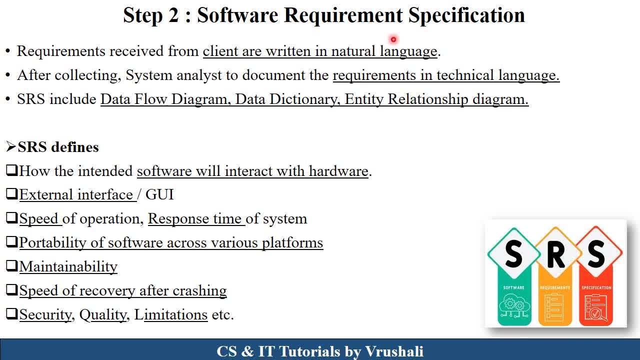 document are called as SRS, that is, software requirement specification. basically all the requirement received from customer are written in natural language like Marathi, Hindi, English in this language, but SRS document are maintained in technical language which is understandable by the implementation team. this SRS document also having different diagrams, like data flow. 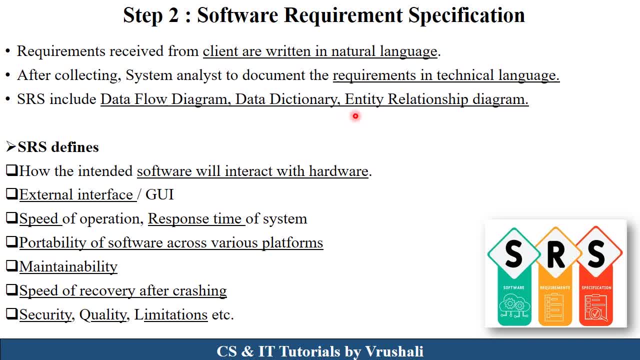 diagram- data dictionary entity relationship diagram. this SRS document also having different diagrams, like data flow diagram, data dictionary entity relationship diagram, they show the work of the particular product now this SRS also include software and hardware requirements related to the project. then external interface GUI, how your product look like in. 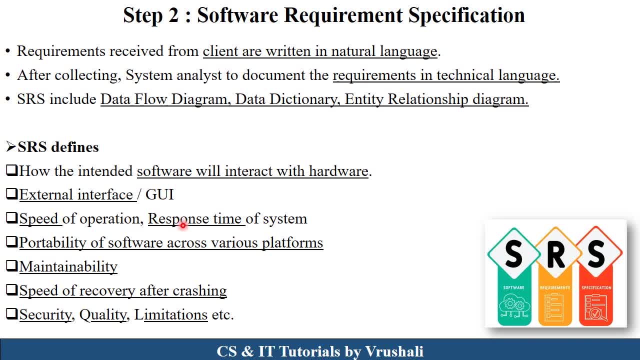 future their diagram: speed of operation, response time of system. then portability means particular product work on different type of operating system like windows, linux. so their portability features: maintain ability, speed of recovery after crashing, their security and maintenance system, security issue quality and some limitations. so this, all things are included into the 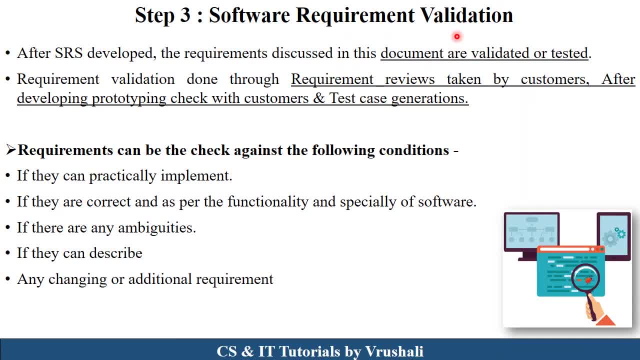 SRS. now the next one is a software requirement validation. after developing SRS document, this document is submit to the customer or each and every stakeholders included in the particular project. now this stakeholder validate the document or test the document. so at that time they take test that if all the requirements are practically implement or it is possible, 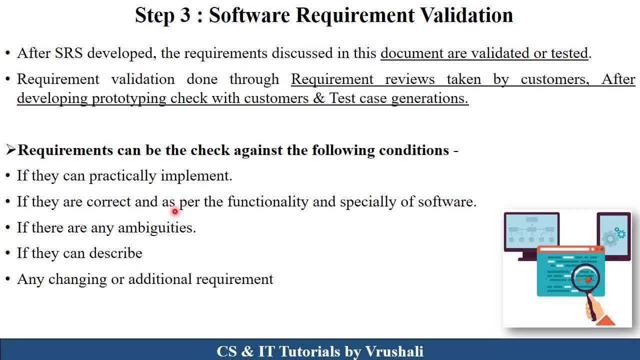 to implement. they test that all the requirements are correctly mention as per the customer ideas, customer requirement. they also check that functionality of the particular software mention in SRS document. if there are ambiguities means if there are any missing information, if they can describe each and every requirements properly or any changing or additional requirements are. 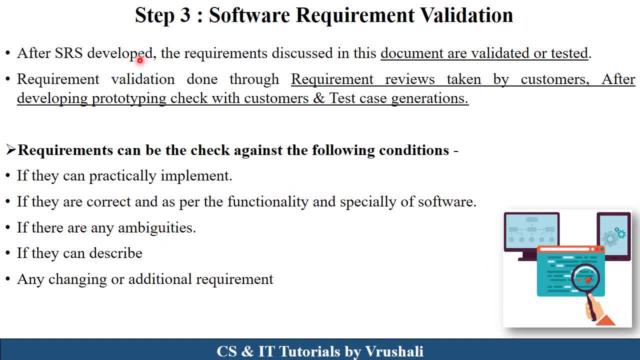 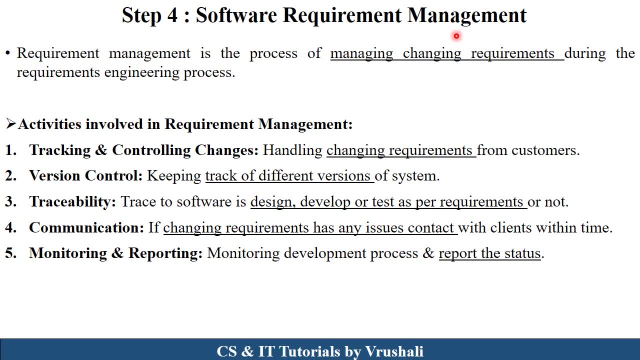 there. so this: all things are validate or test in SRS document. then they maintain the changes in this particular document and send this document to the development team. clear. next, now the last one, is a software requirement management. so here this after requirement management manage all the changing requirements. as we know, we 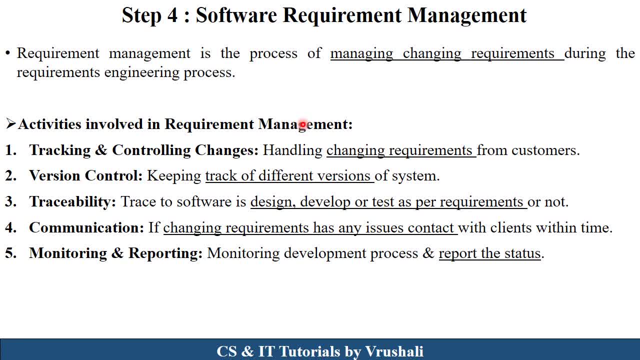 discuss early in sdlc models. customer requirements are continuously changing. at development phase also, customer requirements are changing so it is very important to manage all this changing requirements. so there are different activities involved in this requirement management. the first one is a tracking and controlling changes. here requirement manager handle all the changing requirements from 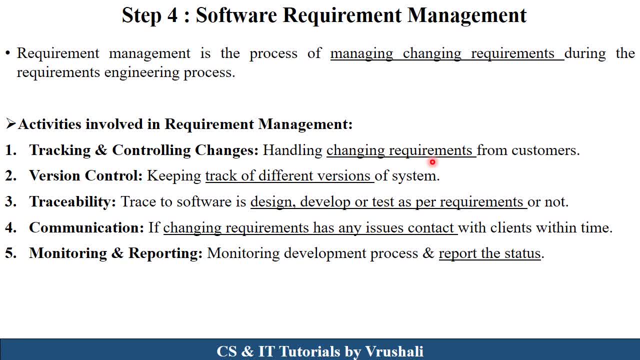 the customer. they take this changing requirements from the customer, communicate with the customer and check that this changing requirements affect on overall system or not. then version control- this the requirement manager keeping track on different versions of system. as we know, suppose whatsapp application, when you update whatsapp there are different features. 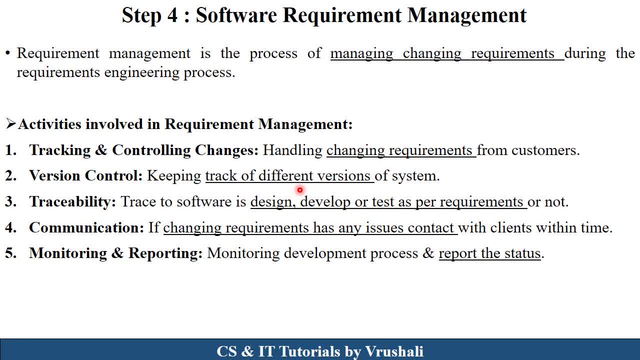 are there, means every monthly, monthly or weekly. there are different features or different versions are there, so keeping track on different versions of system. then traceability: traceability means requirement manager, test a particular software, particular product in each and every phase, like design, develop or testing phase, which it is customer requirement matching. 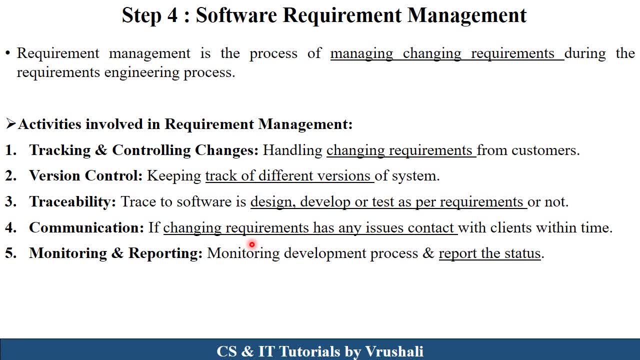 or not. then communication, if customer changing requirements having any issue or which is not possible to implement, so they communicate with the customer regarding this. and last one is a monitoring and reporting means. they monitor complete development process and report the status to each and every stakeholders. clear. next now this is all about requirement engineering process. so these are the some.